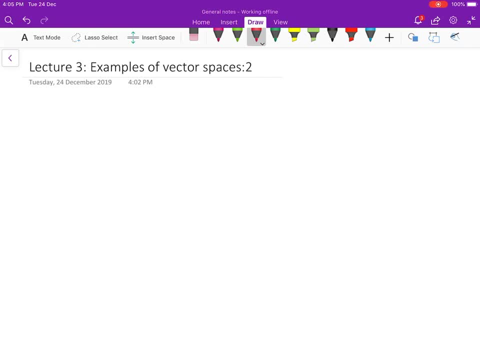 hello everybody, welcome to this next video on vector species. so in the last video we were discussing about the examples of vector species and the first example which we had discussed was RN as a vector space over R, where R denotes the set of all real numbers and RN means n-tuples. so in this video we will look 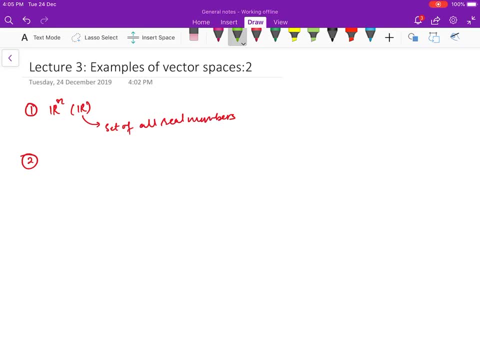 at some more examples so we can have this example which we have done in the last video. we have, you know, checked all the ten properties very nicely, so whenever you have some confusion that how one property should be proved for a particular vector space, you can go back to video 3 right to have an idea in this. 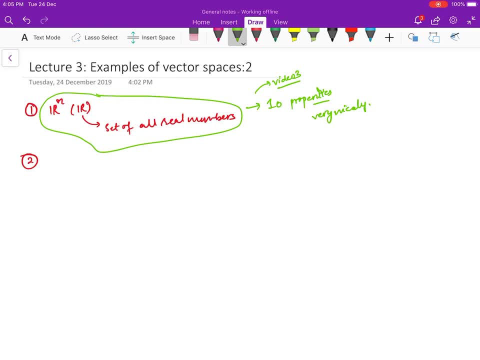 video. I will just brief you about the properties. so the next example which we are going to talk about is C, which is a set of all complex numbers, and R is your field set of all real numbers. so we we have C is a vector space over R, where if you take two elements, u and v- from C, then they look 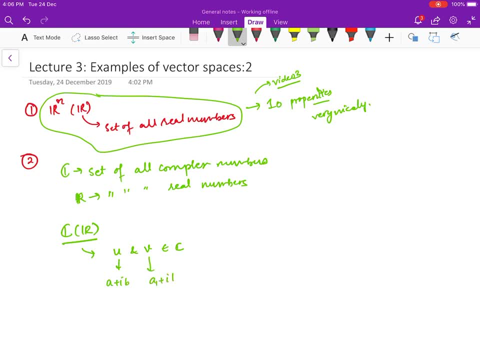 like a plus ieta b and say a1 plus ieta b1. so addition is defined as u plus v is defined as a1, a plus a1 plus ieta times b plus b1. and if you take alpha from R and you take this is from your field, R and u is 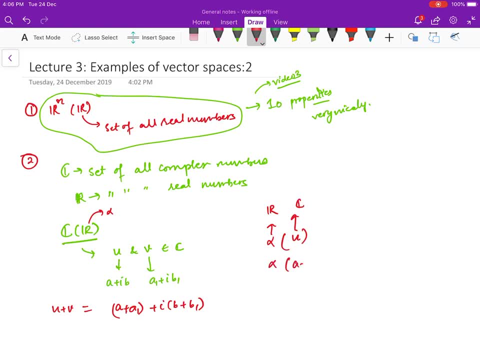 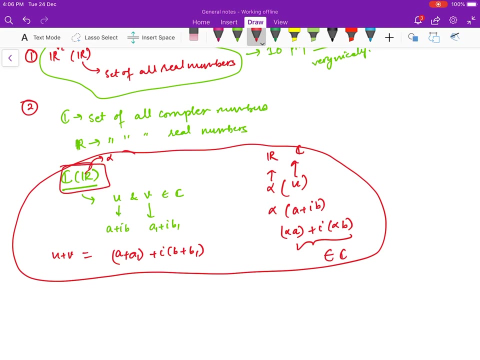 from your set C, then this is alpha a plus ieta b. this is defined as alpha a plus ieta times alpha b. so this again belongs to C, right? so under to these two operations, this is a vector space, right? and you can see that additive identity. 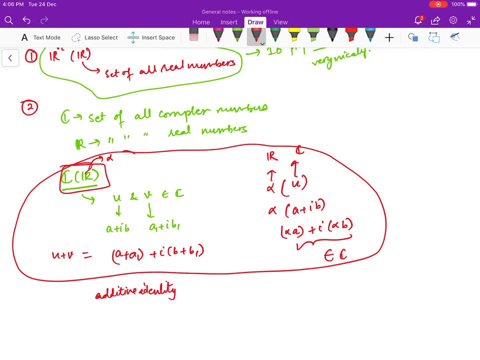 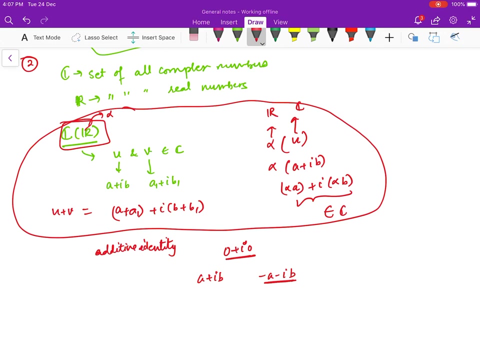 is, is your, as you have to, 0 plus ieta 0. so 0 as a complex number is your additive identity. and for each complex number, a plus ieta b minus, a minus ieta b is also complex number. that is your additive inverse. and then you have all the properties, other property, distributive. 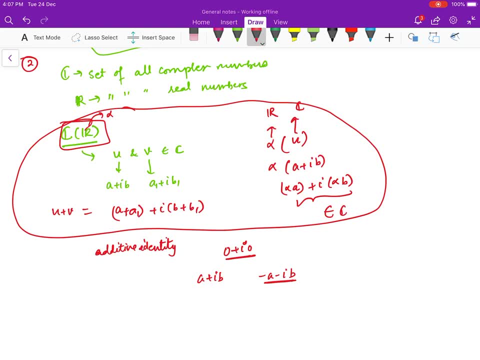 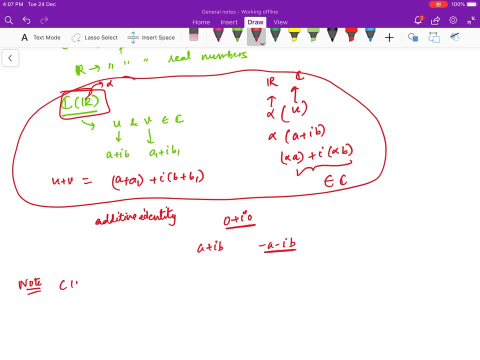 and associativeness and commutativity. everything is there. you can check that. so this is one of the example. and then you should note that c over r is a vector space. but if you reverse it, r over c is not a vector space. why? because if you take alpha from here and then you take a real number, you multiply a complex. 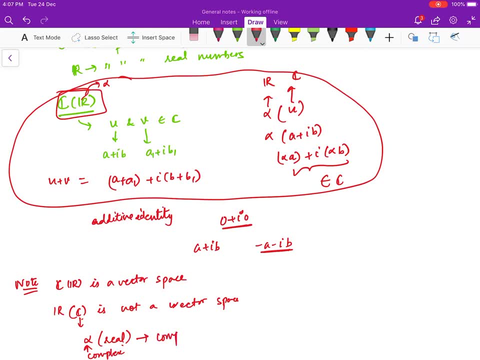 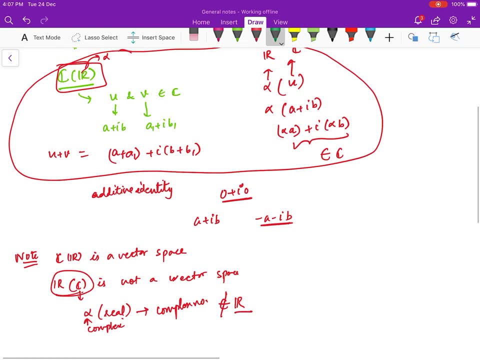 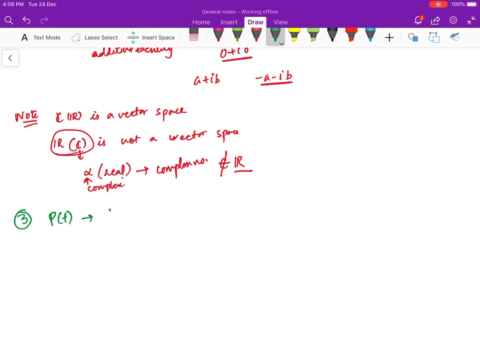 number. with a real number, you are going to get a complex number. so this is no longer in r. so that is why r over c is not a vector space. now let us look at another example. if you take pt, which is set of all polynomials, set of all polynomials. 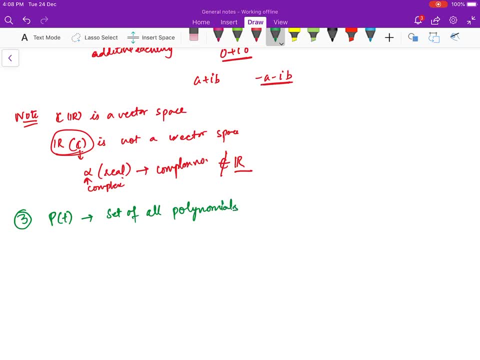 means polynomials of all possible degrees. so here you have constants. like all the constants are there. they are polynomials of degree 0. then you have a plus bt, where a and b can be any real numbers. so you can see, it is a set of all polynomials with coefficients from r. actually you can. 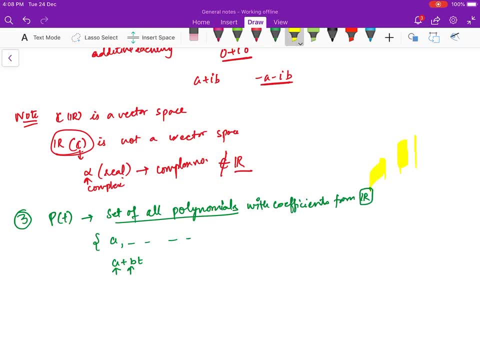 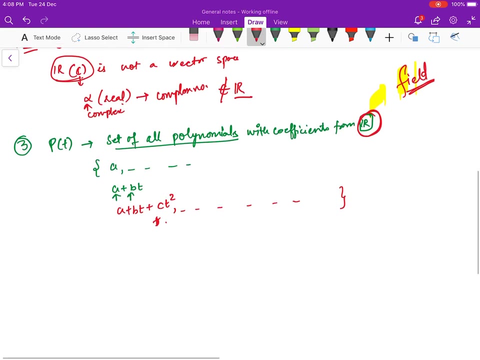 generalise it here. in place of r you can have a field, any field will also work, but right now we will take that coefficients are real numbers. so then you have polynomials of degree 2 also, and degrees, degree 3 also, and so on, so it contains polynomials of all possible. 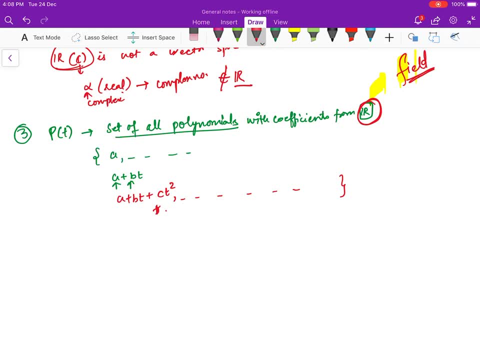 degree right? so you can see that Here the operations plus operation is defined as if you take two polynomials, pt plus qt, you add the constant terms, and then you add the first degree terms, and so on, Add the second degree terms, and so on. 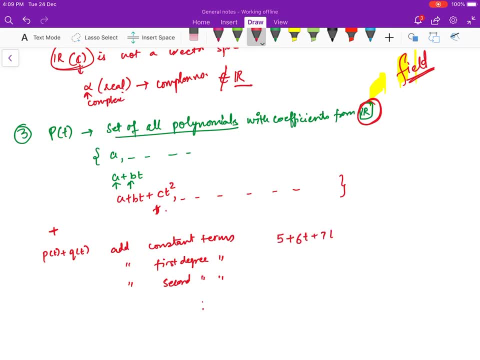 For example, if I give you 5 plus 6t plus 7t square and another polynomial is say 6 plus 5t minus 3t square plus 5t cube, then you will add 5 and 6, you have 11. you will add 6 and 5, you will have 11t. then you have t square here minus 3t square. here you have 4t square. here is 0t cube, here you have 5t cube, so you have 5t cube. 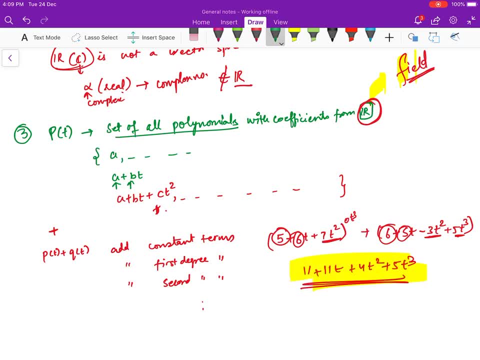 So like this you are going to proceed. So this is how the sum is defined And pt is your set and r is your field. If you take a number, alpha, from r and you multiply pt, it's like alpha say this polynomial is a naught plus a1t plus. so on a n, t raised to power n. 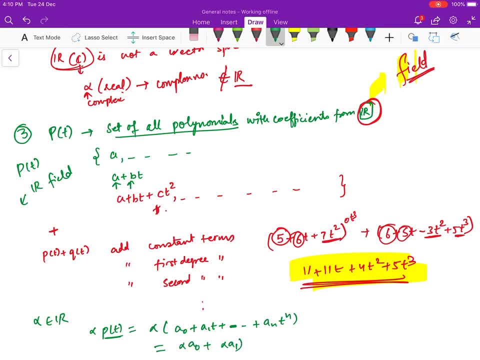 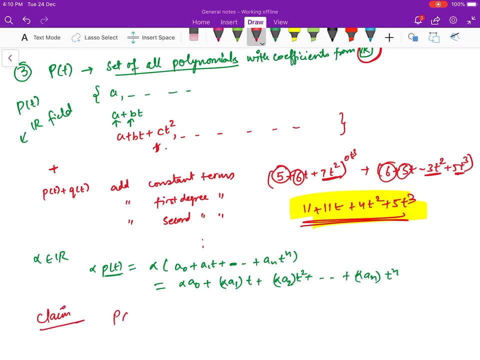 So this is equal to alpha a naught plus alpha a1 into t, plus alpha a2 into t square, and so on. alpha a n into t, raised to power n. So this is how the two operations are defined And the claim is that pt, which is set of all polynomials, is a vector space over the field r. 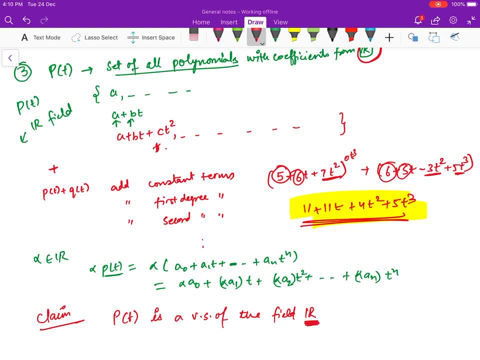 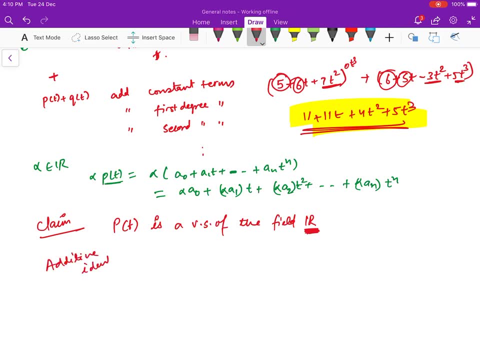 It is actually a vector space over the field. from wherever you are taking the coefficients Here, what is your additive identity? Zero element. So that is your zero polynomial. So we will take pt equal to zero. This is your zero polynomial Right. 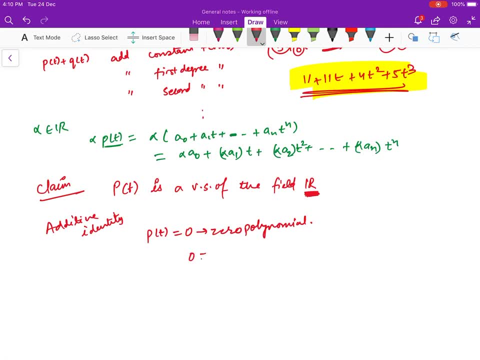 So the degree of this polynomial is not Defined, because you can write zero as zero. You can write zero as zero plus zero t. You can write zero plus zero t plus zero t square. So you can write in any form. So degree of this polynomial is generally not defined. 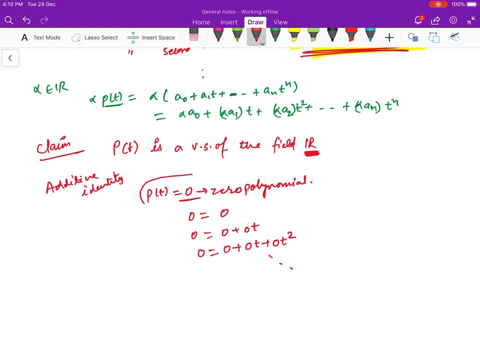 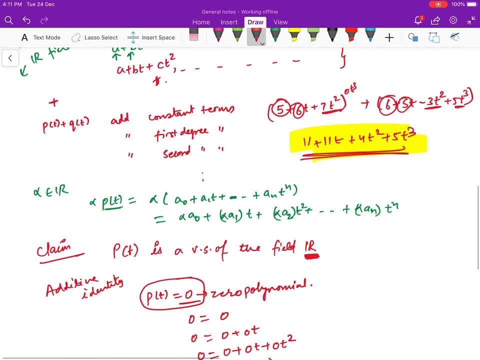 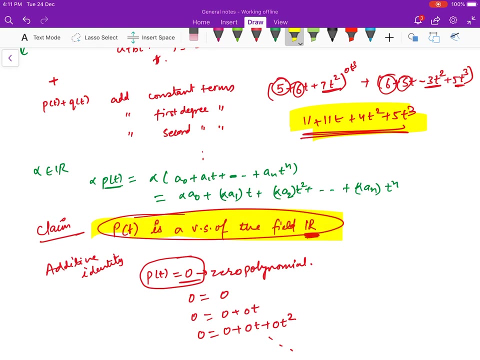 But this is a polynomial. It is included in the set of all polynomials, So this will work as your additive identity And all other properties. you can easily verify that they follow. So that is why pt over r is a vector space. So this thing, we can note that pt over r is a vector. 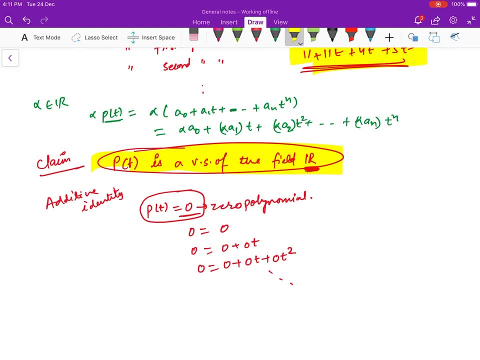 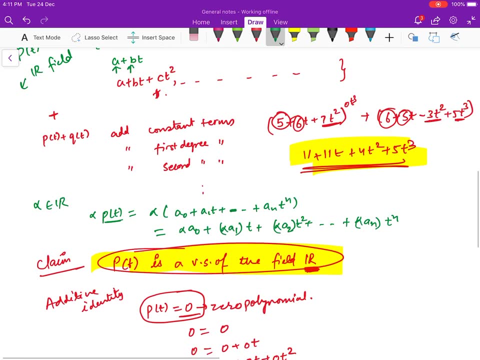 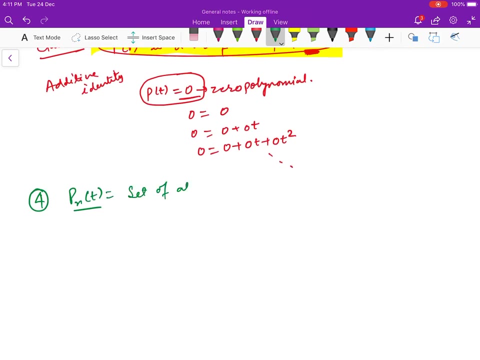 Now let us look at some more examples. So the next example is: You can have p and t Here. we had taken pt set of all polynomials. We can restrict this set, So we have p and t's set of all polynomials. 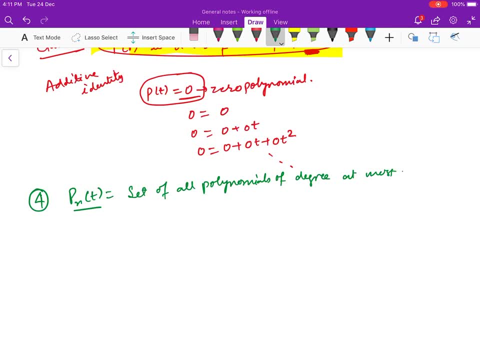 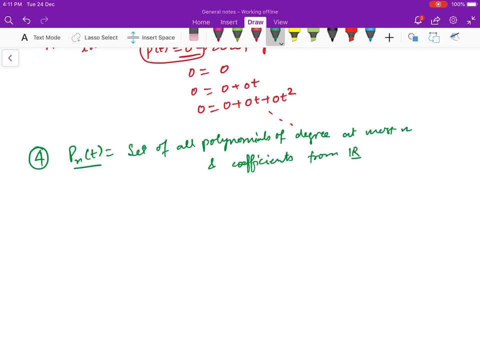 Of degree, at most n And coefficients from r The field, then p and t Right. This is actually a set of this form: A1, a naught plus a1t plus a2t square, and so on. a and t raised to power n.